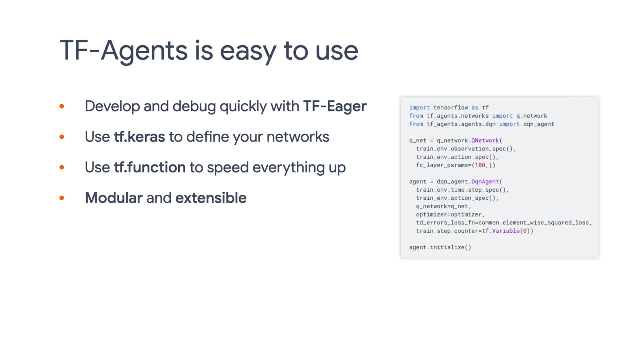 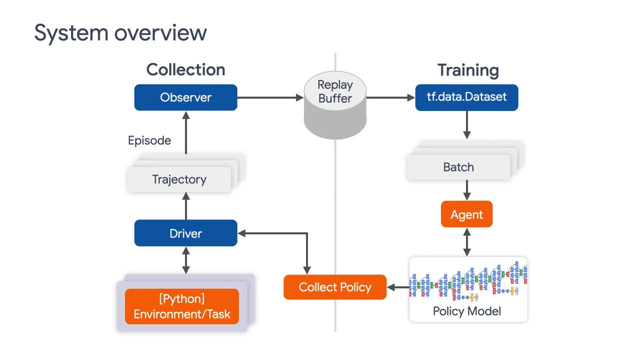 TF Agents is also modular and extensible. You can easily set up a RL environment or agent quickly. Lastly, our extensive examples and documentation can help you get started really fast. Here's an overview of TF Agents components At a high level. the process to train a RL agent is: 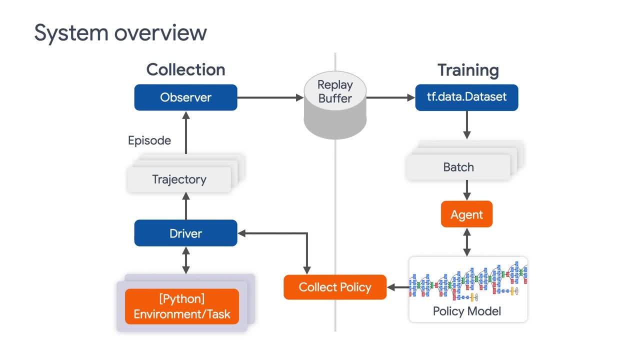 We use our agent to interact with the environment so that we can collect experience trajectories. We then feed the trajectories to our agents to train it so that it becomes better to receive the rewards. We keep doing this until the agent has good policy to extract the most rewards from the environment. 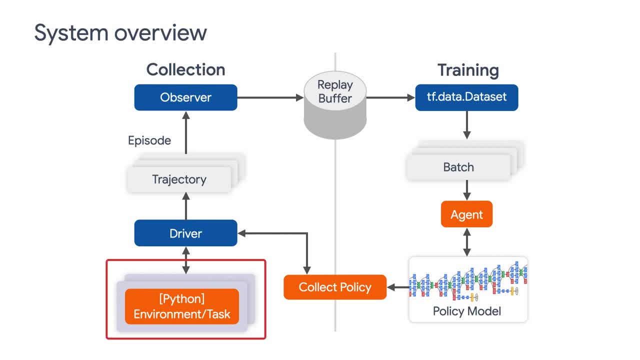 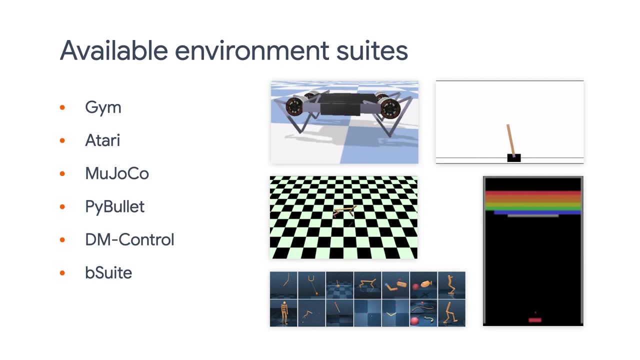 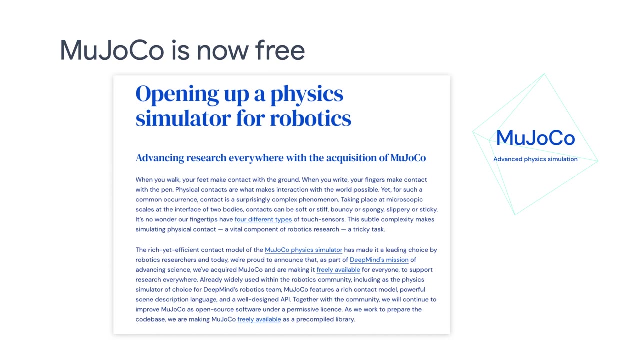 Let's talk a little bit more about environments and agents. First, the environment TF Agents supports a wide variety of environments: GIMP, Atari, PyBullet, DeepMindControl and B-Suite TF Agents also has an interface to Mujuko. 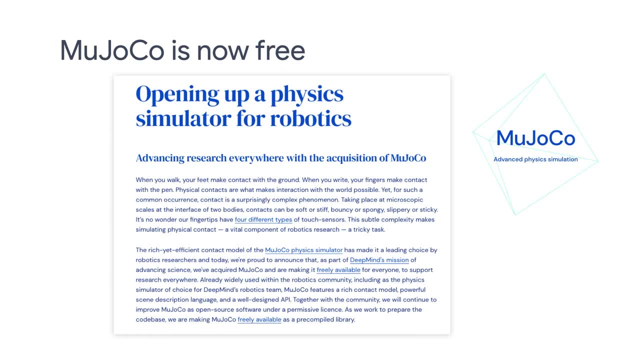 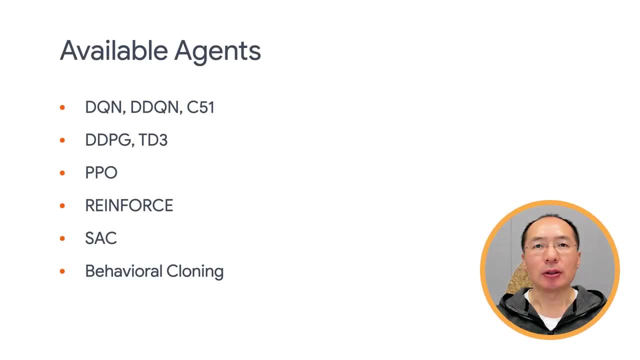 Recently, Mujuko was acquired by DeepMindControl. It is now free to use Next agents. TF Agents has implemented a number of classical and state-of-the-art agents, such as DQN, Reinforce and PBO. They are fully tested and ready to use as black boxes. 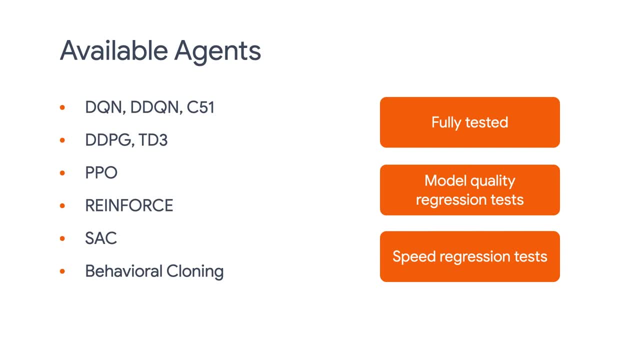 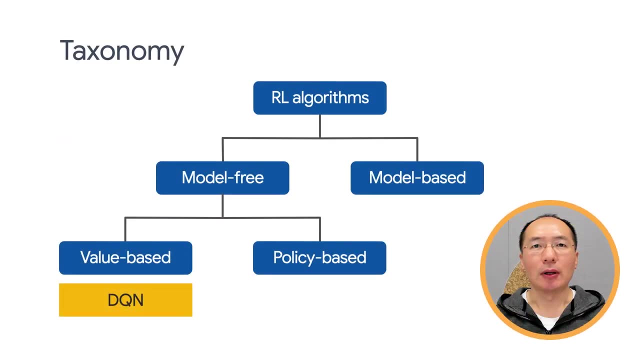 That's the nice thing about TF Agents: You don't necessarily need to know how to implement these agents yourself, but you can still use them effectively for your own needs. Now let's walk through an example of using TF Agents. This is a DQN agent with TF Agents. 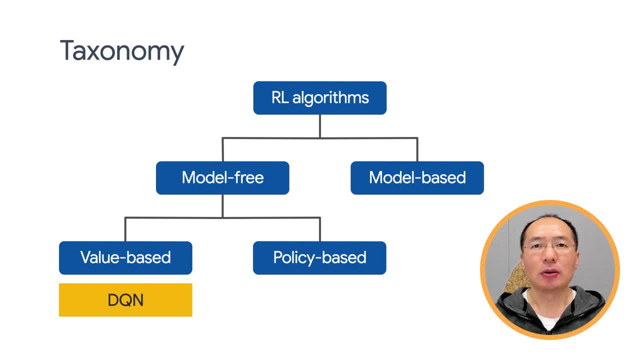 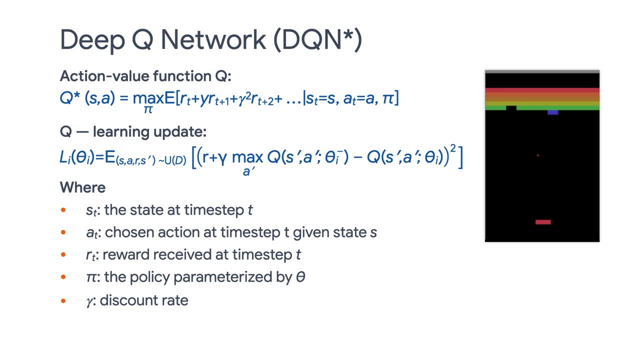 Remember that DQN is a kind of value-based method. You'll see why in a minute. DQN stands for Deep Queue Network. Here Q is what we call action-value function. It basically means if the agent is in state and is going to take action. A. 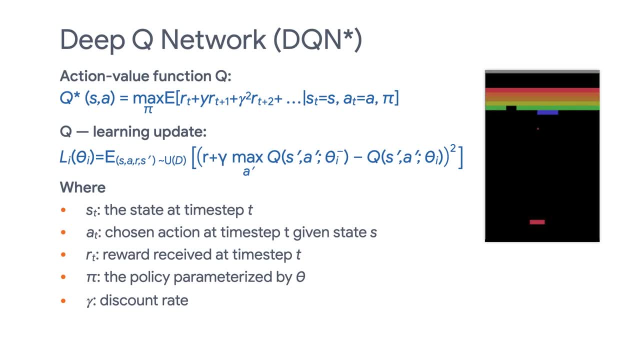 what's the expected total reward for that action over the time horizon And the optimal action-value function? Q-star gives the best value possible from any possible value policy, which is the first equation. So think about this Intuitively if you know the reward. 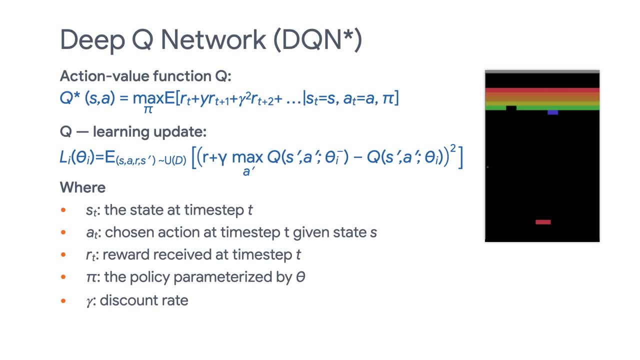 values for all possible actions. given a state, it's pretty easy to pick the best action for that state. right Now, our job is to represent the Q function with a neural network which leads to the second equation. We're not going into the math here, but basically it tells you how to update. 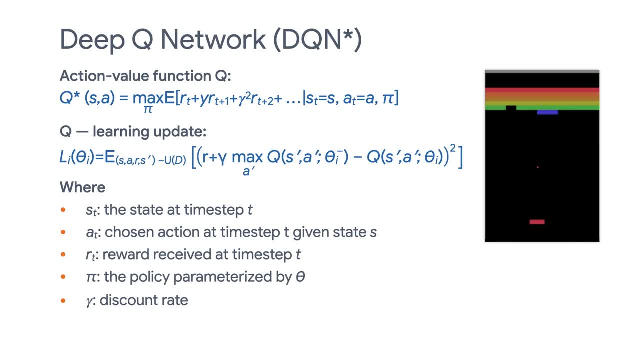 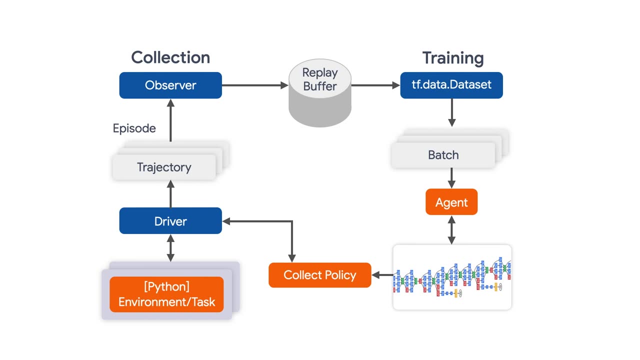 the neural network parameters based on the experience trajectories we collect during the training gameplays. For a more detailed discussion on DQN, I highly recommend the reinforcement learning course by DeepMind and University of College London. Now we come back to this overall picture of TF agents For the environment. we're going to use the built-in CardPro environment. 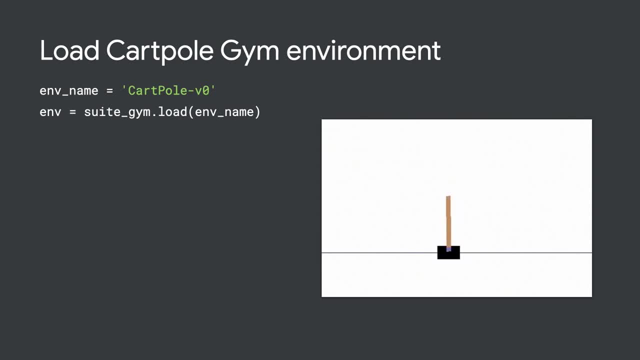 TF agents provide an easy interface to load environments from GIM. We just call load function here And TF agents will take care of it. We call that. we're trying to keep the pole balanced by moving the card left or right. The agent receives a reward of positive one if the pole 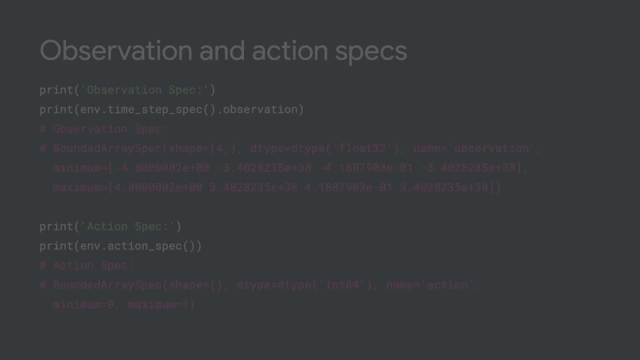 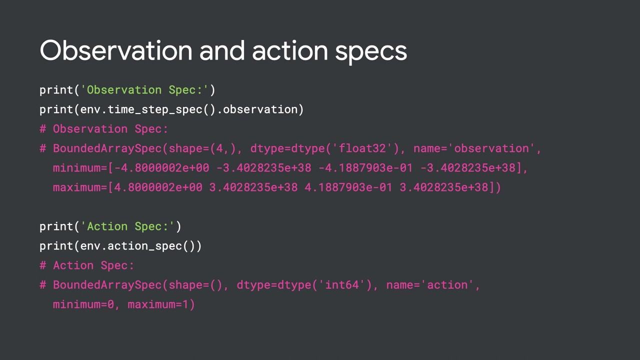 remains upright at each time step. It's important to understand the environment specifications, since not all agents are compatible with all the environments. Here we print out the specs of the observation and action. You can see that our observations is a tensor of four float values, which are: the card's position, velocity, the pole's angle. 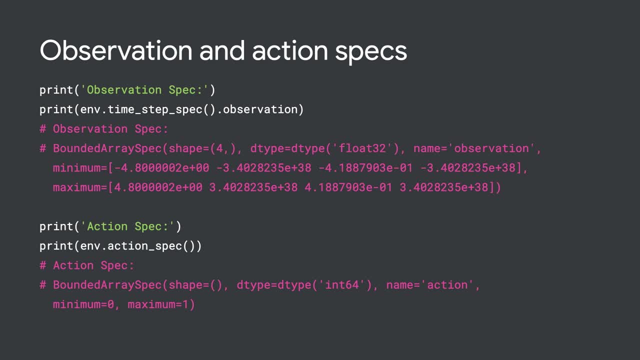 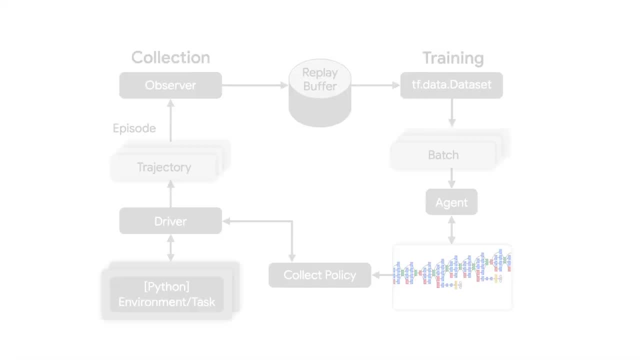 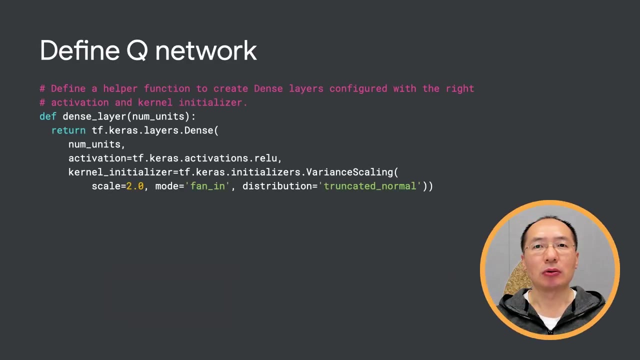 and velocity respectively. The action is just an integer that can be zero or one, which means we move the card left or right. Now we define our queue network. As I mentioned just now, we're going to use a neural network to represent the queue function. 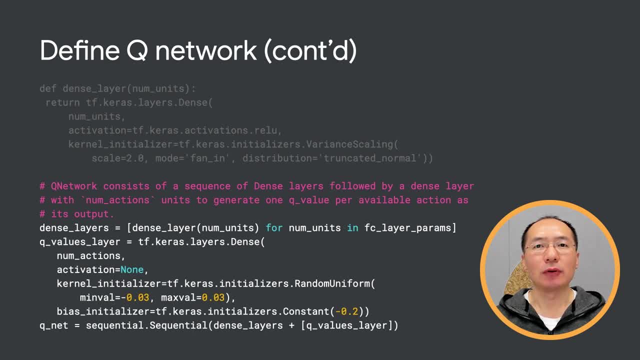 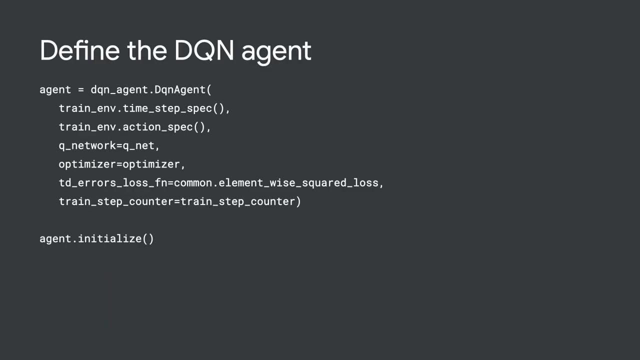 The network is pretty simple and consists of a few dense layers. The last dense layer needs to output a probability distribution over all possible actions, which then allows us to pick the best action. We stack all layers together and we have our queue network. Next we define our DQN agent. We basically pass the environment, specs and queue. 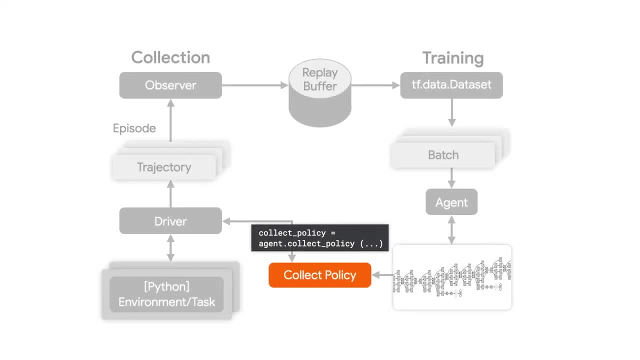 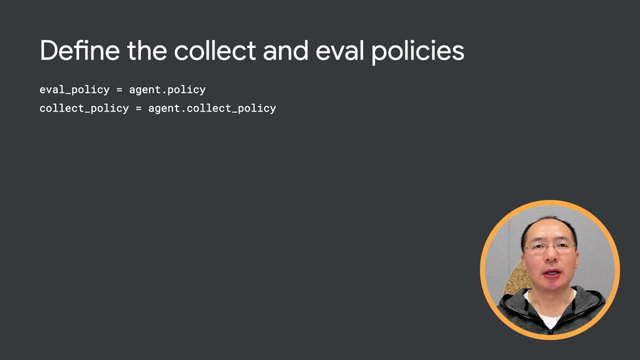 network to the DQN agent. Next, we define how we collect the experience trajectory. All agents contain two policies. Agent dot policy is a policy that is used for evaluation and deployment. Agent dot collect policy is a second policy that is used for data collection. 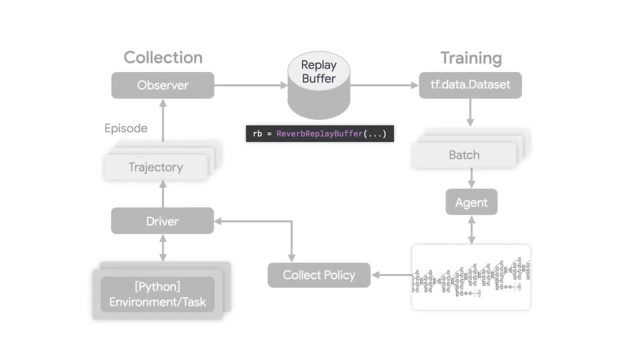 In the original Atari DQN work by DeepMind in 2015,. there's a technique called experience replay to make the network updates more stable. Basically, at each time step of data collection, the transition data are added to a circular buffer called the replay buffer. Then, during the training, instead of using just the latest, 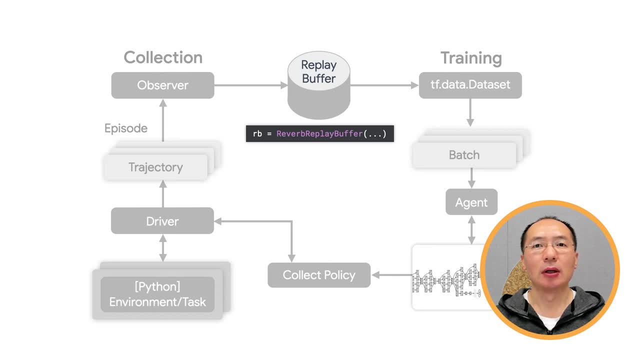 transition to compute the loss and the gradient. we compute them using a mini-batch of transitions sampled from the replay buffer. This has two advantages: Better data efficiency by reusing each transition in many updates, and better stability using unrelated transitions in a batch. 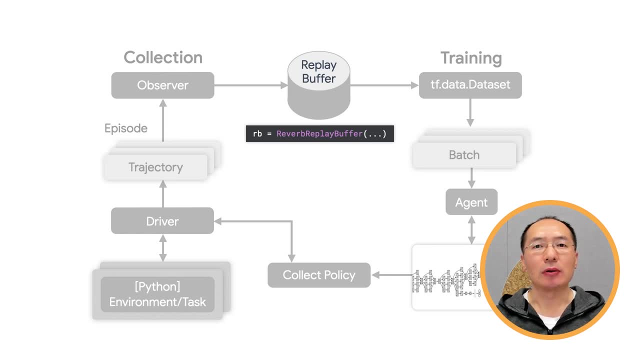 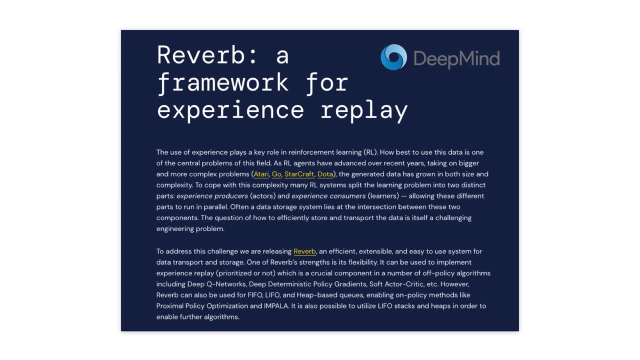 We also call these transitions trajectories. We'll see how these trajectories look like in a minute. To store and sample these trajectories for training, we set up a replay buffer. We're going to use a framework called Reverb. It is open-sourced by: 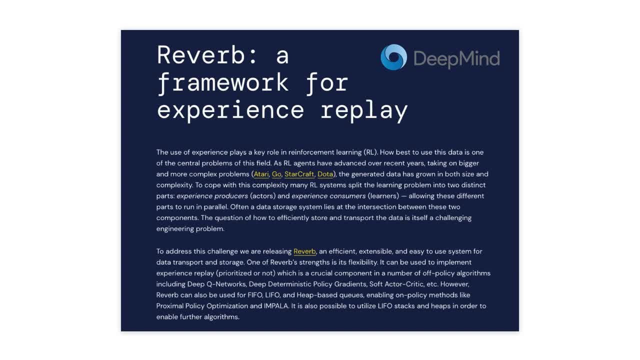 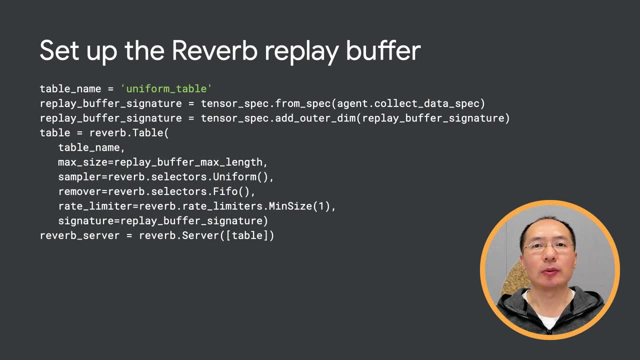 DeepMind and is specifically designed as an efficient framework for experience replay. To set up the Reverb replay buffer, we first create a Reverb table using trajectory specs, sampling rules and et cetera. Then we set up a reverse table using trajectory specs, sampling rules. 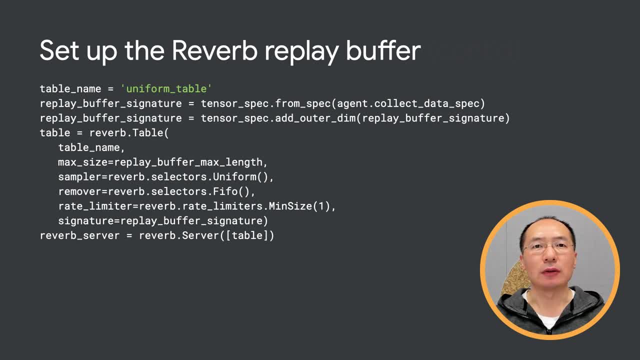 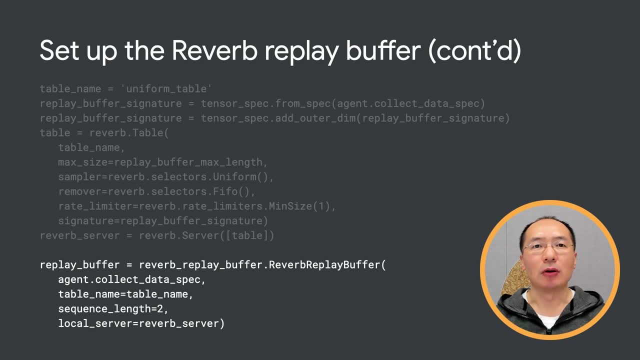 and et cetera. Then we set up a reverse table using trajectory specs, sampling rules and et cetera. We start a Reverb server. Next we create the Reverb replay buffer using the Reverb server and the table. Note that we set sequence length to 2, since this is required by DQNAgent. 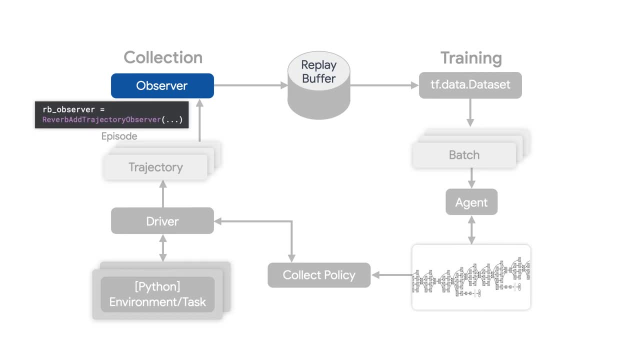 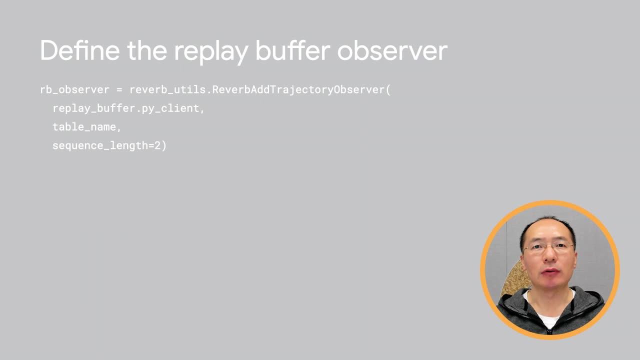 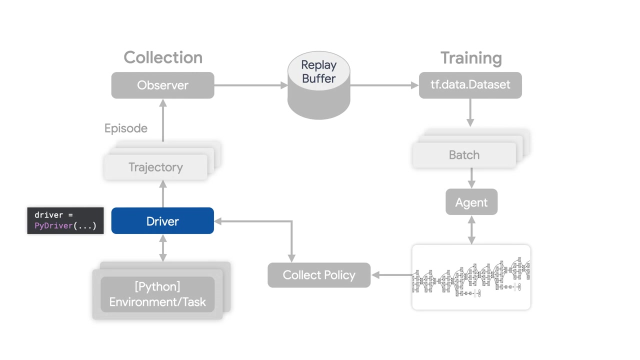 Now we create an observer to the replay buffer. We create a replay buffer observer here. It will be added to the driver in a minute so that the trajectories can actually be collected into the replay buffer during the training. The last piece of the puzzle is driver. Driver is a utility that runs the experience collecting. 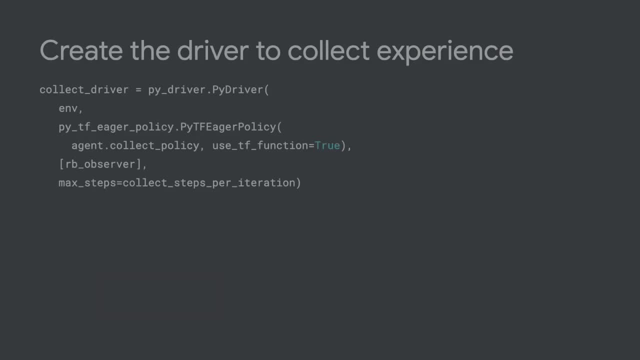 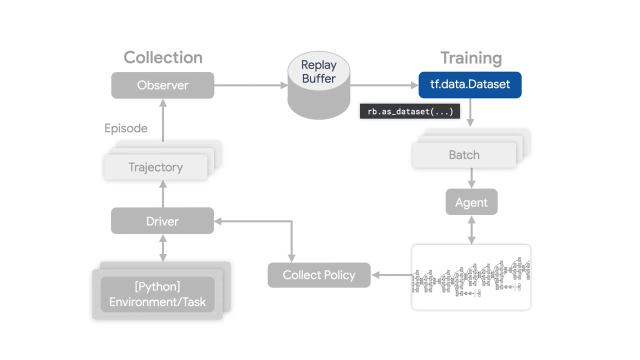 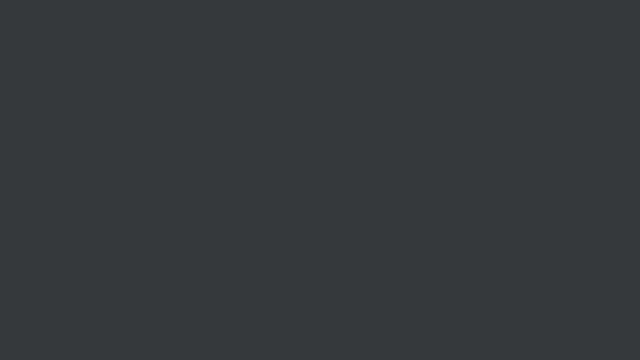 loop for a certain number of episodes or steps. We pass our replay buffer observer to the driver to collect trajectories for training. After training data is collected into the replay buffer, we can sample them out as a TF dataset. Here's how our experience trajectories look like. It contains: